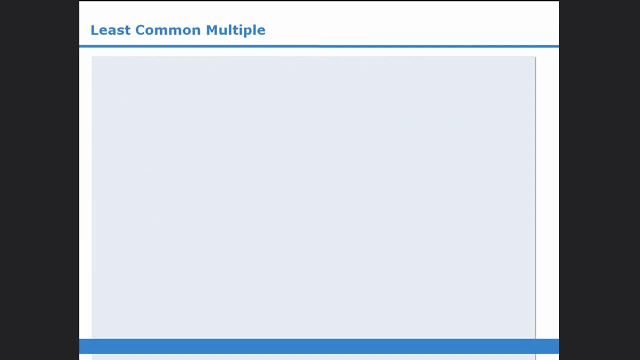 Now let's examine another technique for finding the least common multiple. To demonstrate this technique, we'll find the least common multiple of 12 and 56.. For this technique, we'll first find the prime factorization of 12, and then we'll find the prime factorization. 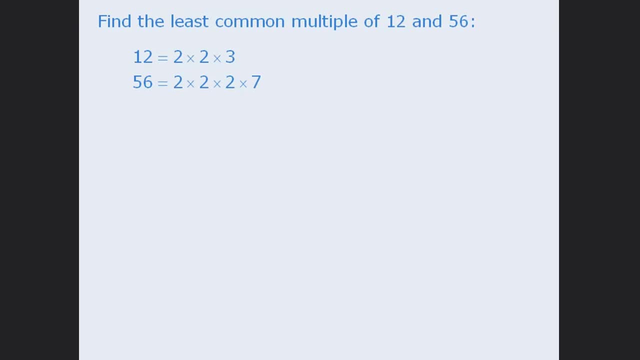 of 56.. At this point we'll find all of the prime factors that they have in common. Now they both will leave 12, so we'll find a pair of twos and another pair of twos, So we'll note that here. 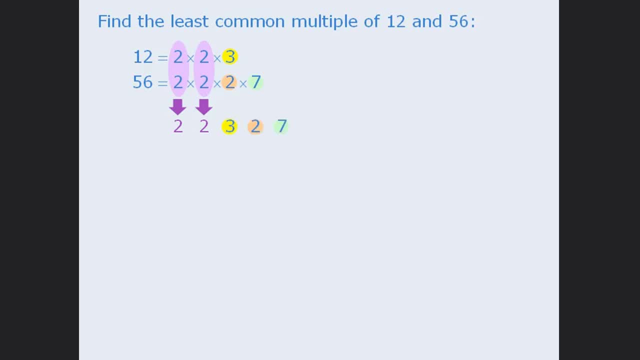 Now we'll take each of the prime factors remaining and list them with the two common prime factors. At this point, the least common multiple will be the product of these numbers, which is 168.. Let's try another example. Let's find the least common multiple of 18 and 42.. 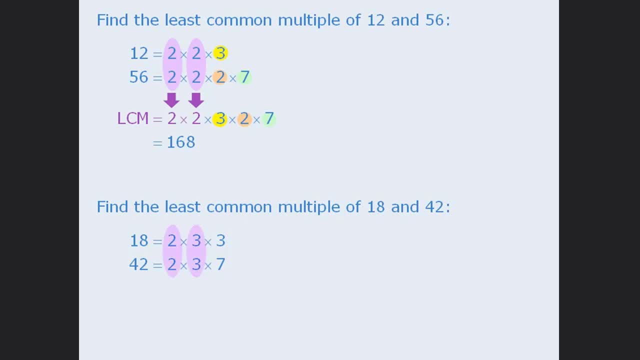 So first we'll find the prime factorization of each number, Then we'll note the prime factors that the two numbers share, Then we'll take all of the remaining numbers and include them in our list. Finally, the least common multiple will be the product of these numbers. 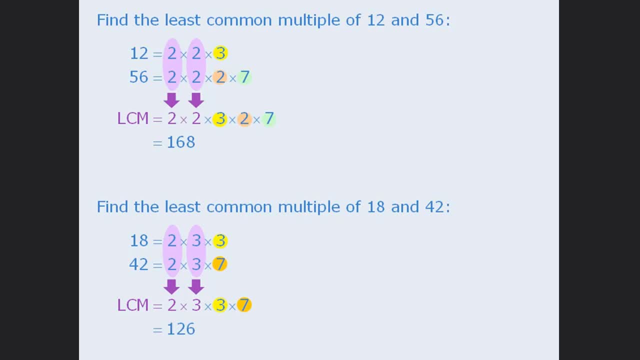 So the least common multiple of 18 and 42 is 126.. So that's the systematic way to find least common multiples. Now that you know two ways to find the least common multiple, you may be wondering when you will ever need it. 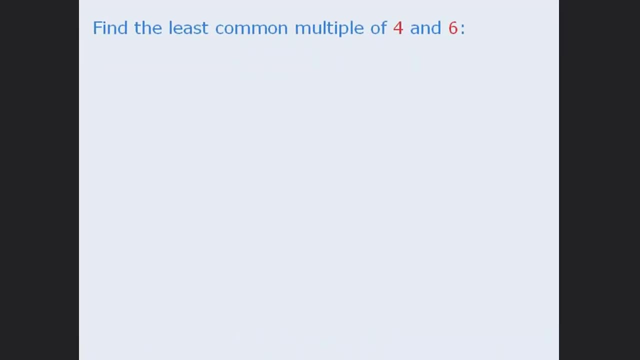 For example, under what circumstances would we ever need to find the least common multiple of 4 and 6?? Well, one situation is adding and subtracting fractions, For example. if you want to add these two fractions, you will need to first rewrite them using the same denominator. 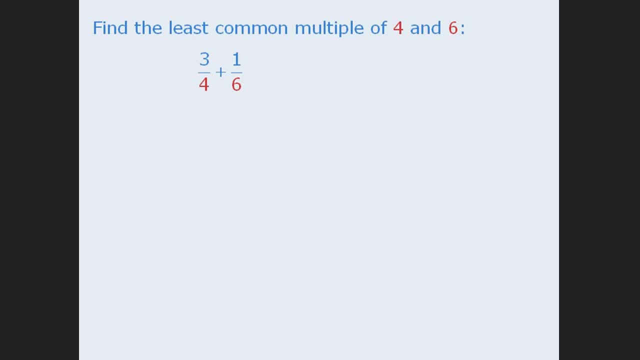 So we're now looking for the smallest number that 4 and 6 both divide into. That number is 12,, so we can rewrite our two fractions with denominator 12.. In this case, we'll use the denominator 12.. So we're now looking for the smallest number that 4 and 6 both divide into. 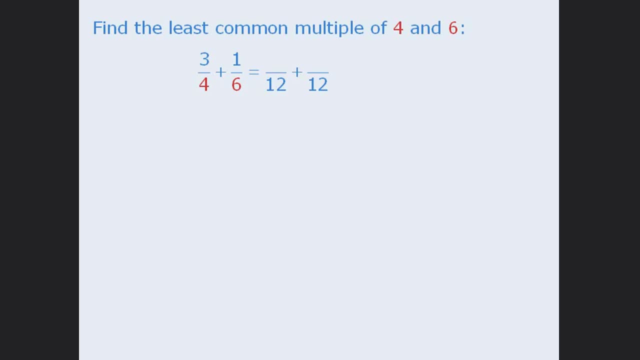 That number is 12, so we can rewrite our two fractions with denominator 12.. In this example, 12 is the least common multiple of 4 and 6.. However, in situations involving fractions, it is usually referred to as the lowest common denominator of 4 and 6.. 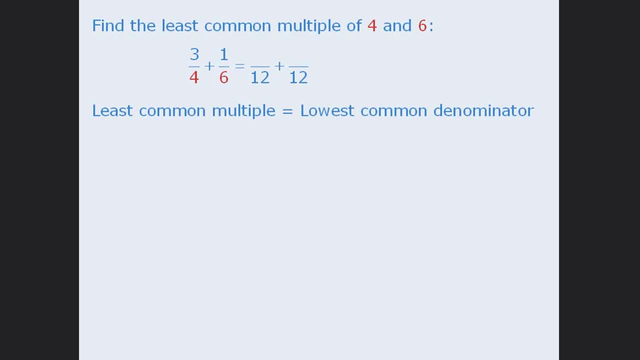 Just remember that both terms mean the same thing. So once we have the lowest common denominator, we can create two equivalent fractions and then combine them. Now, to become an expert on least common multiples, you will need certain skills. First, you must be able to find the least common multiple of 4 and 6.. 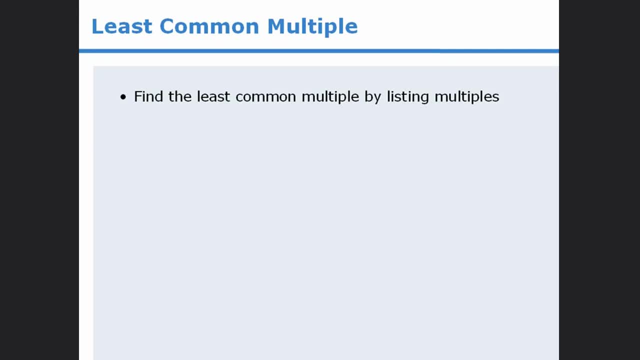 Second, you must be able to find the least common multiples. by listing multiples, as we did at the beginning of this lesson, You should also be good at finding least common multiples in your head. For example, in your head you should be able to identify that the least common 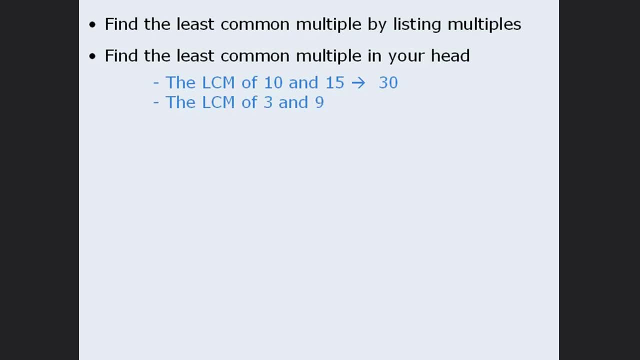 multiple of 10 and 15 is 30. Or, the least common multiple of 3 and 9 is 9.. Or how about 2 and 7?? Well, here the least common multiple is 14.. Another important skill is the ability to find the least common multiple of 7 and 8.. 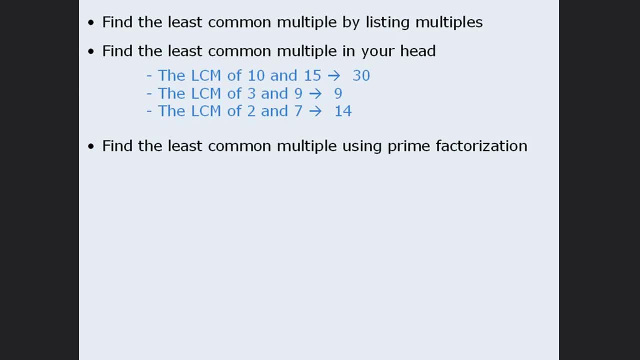 And finally, you should be good at finding pairs of numbers that have a certain least common multiple. And finally, you should be good at finding pairs of numbers that have a certain least common multiple. For example, what are two numbers that have a least common multiple of 18?? 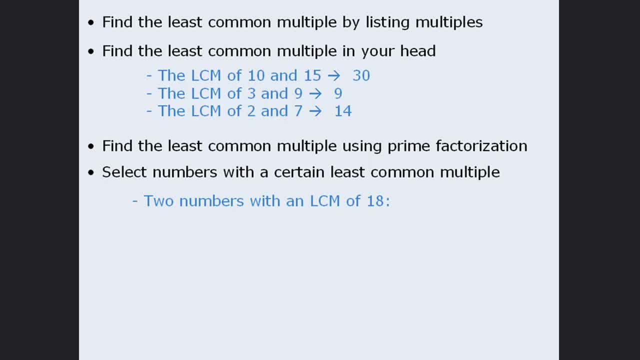 Well, there are several pairs of numbers that meet this condition. They include 6 and 9,, 9 and 18,, 18 and 18, as well as 1 and 18.. Plus, there are many more. Okay, now let's look at some more examples of least common multiples. 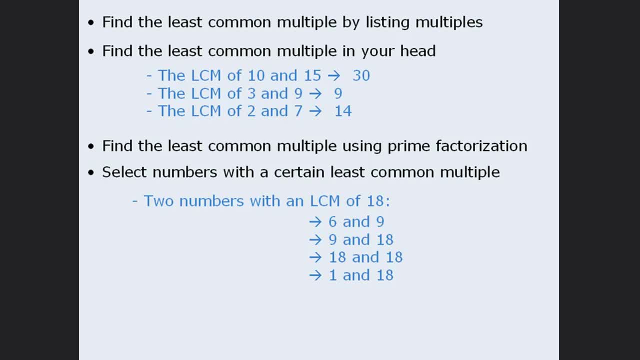 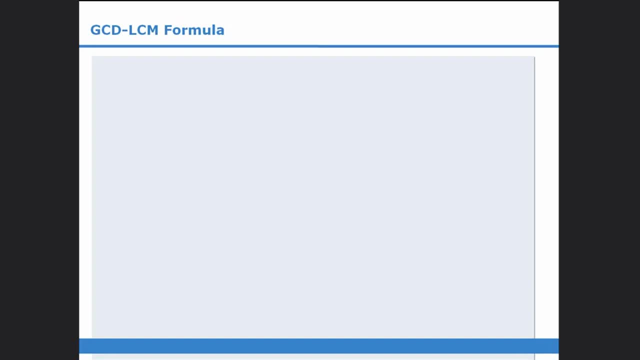 Okay, so these are the skills you will need if you want to master questions involving least common multiple. In this lesson, we'll examine a formula that shows the relationship that exists between the greatest common divisor and the least common multiple of two numbers. To demonstrate this relationship, we'll find the greatest common divisor of 18 and 42,. 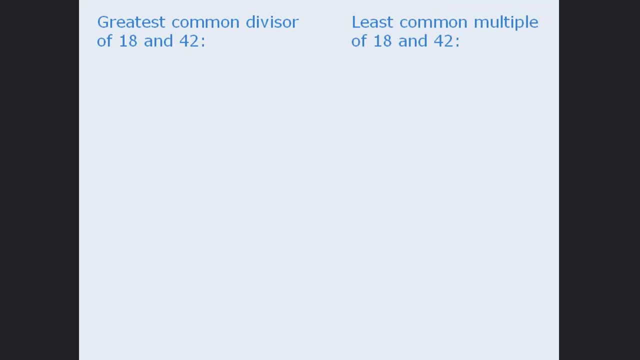 and we'll find the least common multiple of the same two numbers. In both cases we'll use the prime factorization formula. So we'll begin by finding the prime factorization of both numbers and then we'll find all of the prime numbers that they have in common.